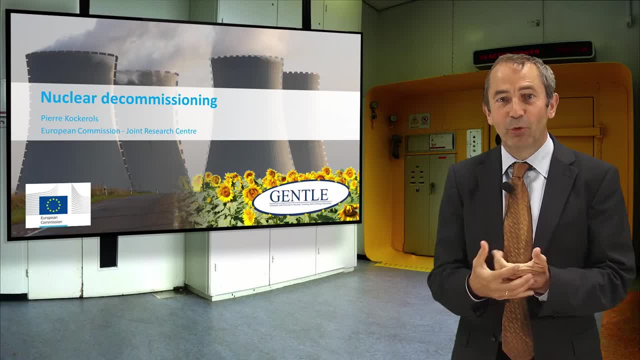 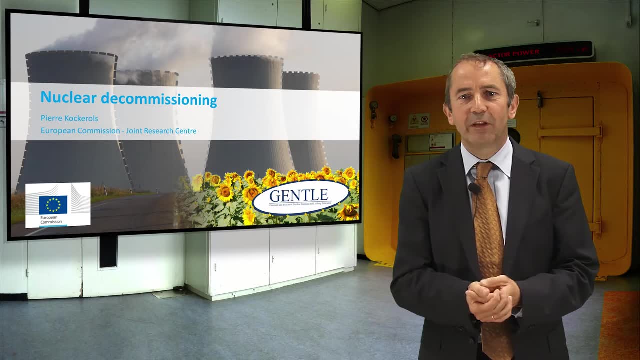 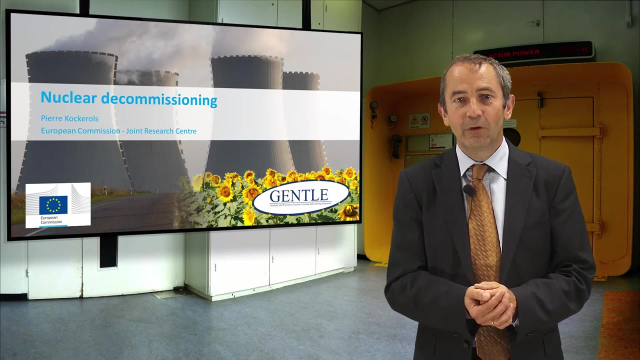 Hello, I'm Pierre Cockerels and I'm working at the European Commission's Joint Research Centre. My lecture will cover a topic that receives more and more attention today: nuclear decommissioning. I will explain you what decommissioning is, why it is important and what the main challenges are for Europe. 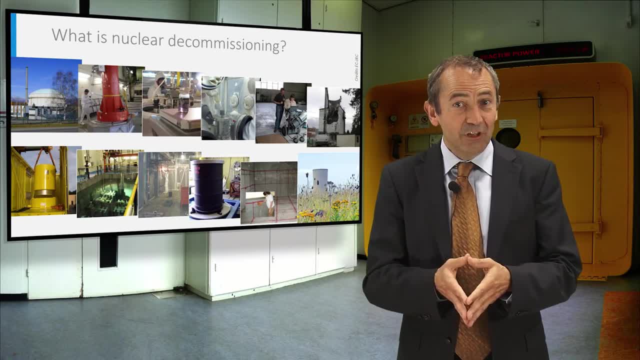 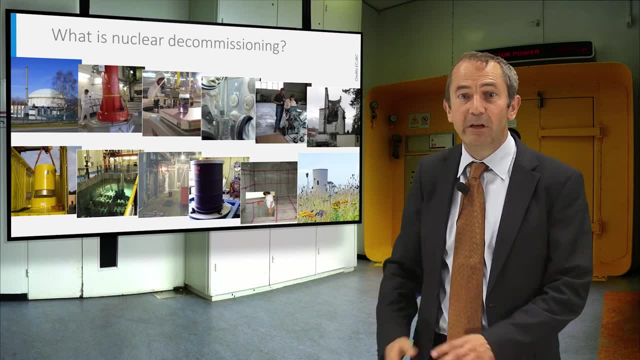 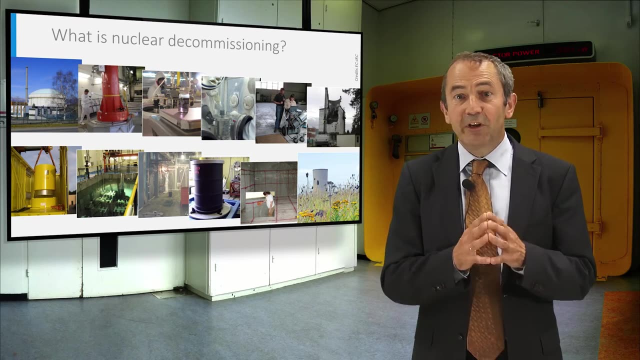 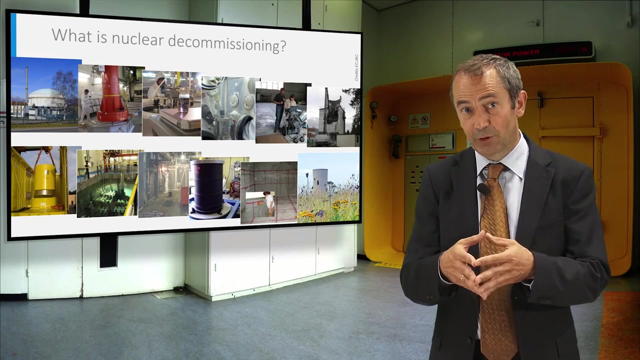 When we speak about nuclear decommissioning, we mean basically all the actions from seizing the operation of a nuclear installation, the preparation of a plan and license, the evacuation of the residual fuel, the decontamination and dismantling, the segregation of the various types of waste, the radiological survey of the buildings and their demolishment if they are not reused. 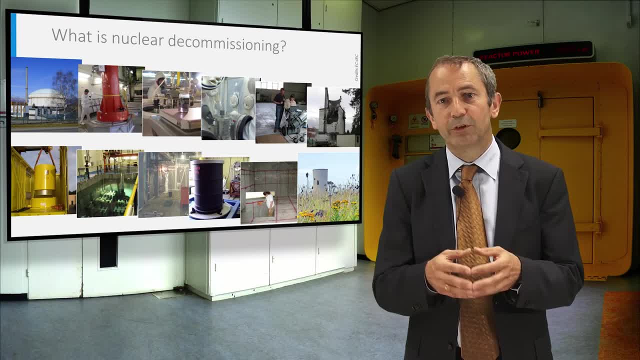 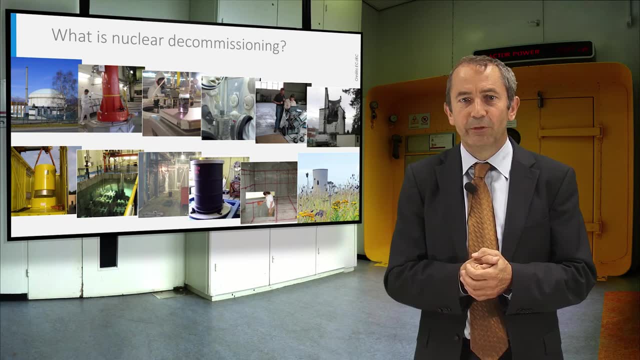 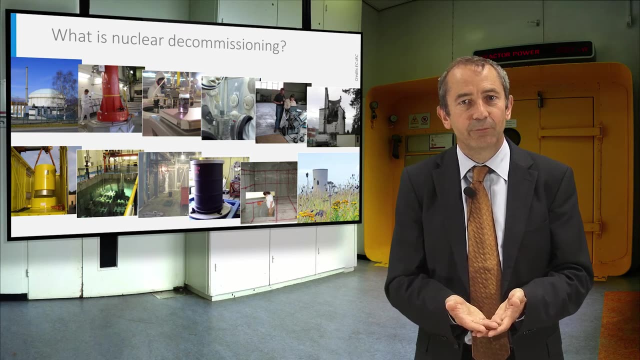 until the final release of the site from regulatory control. Experiences with decommissioning date from the earliest stages of the nuclear history, which, as example, the shipping port reactor decommissioned in only five years in the 1980s, But the practice has gained importance over the last decades. 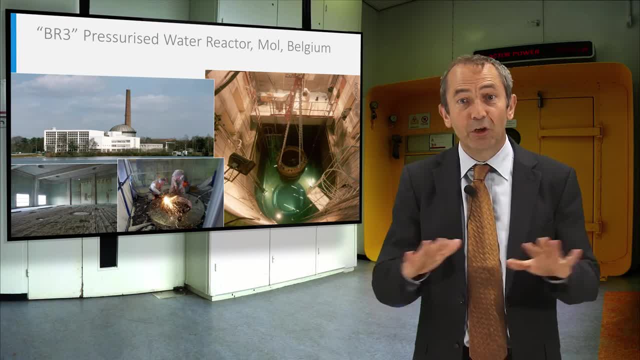 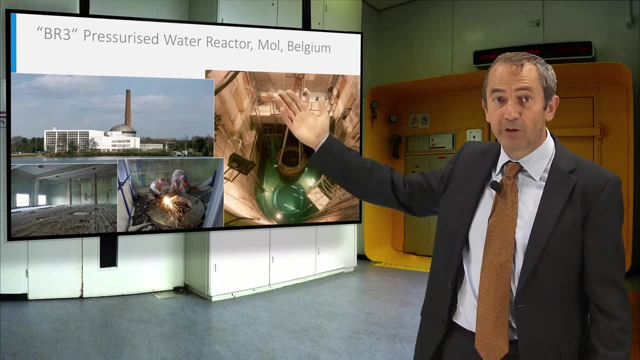 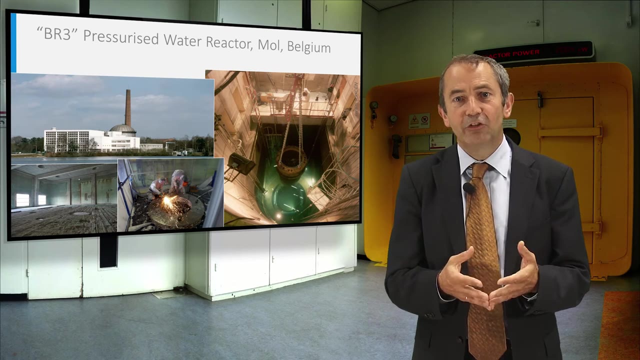 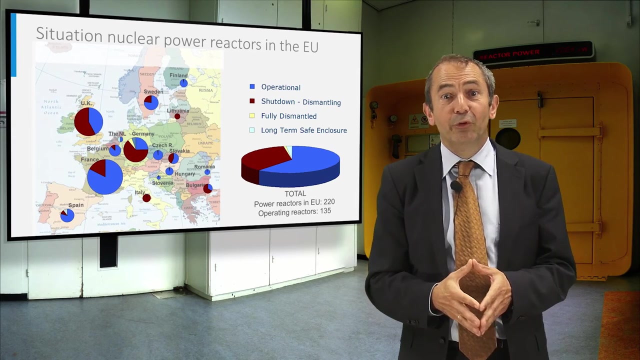 Several EU countries have decided to decommission their oldest facilities. Some first pilot projects were managed under research programs, like nuclear decommissioning, Like the BF3 reactor in Belgium, But currently the activity has grown and reached an industrial scale. A map of Europe shows that about one-third of the nuclear power reactors are currently shut down. 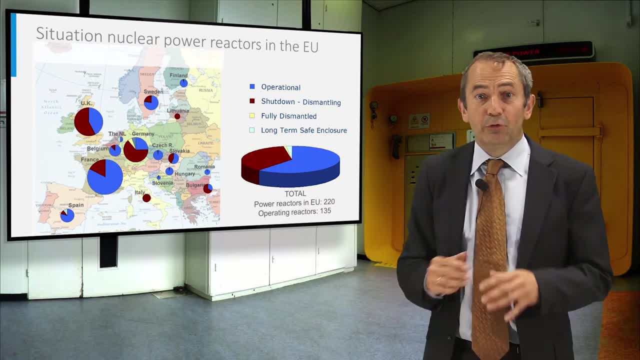 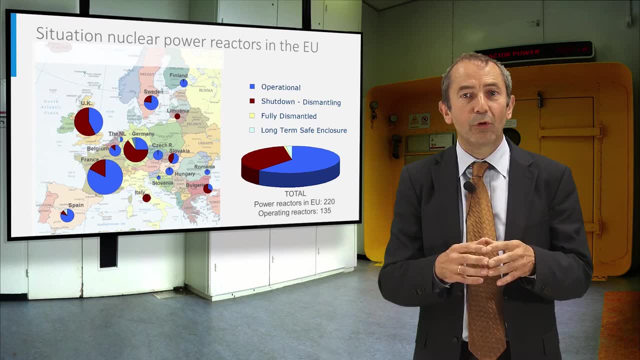 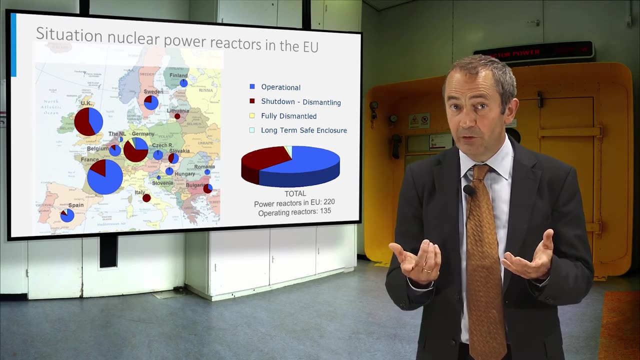 The situation is variable between the different countries. The complete work, from the end of operation until the final release from regulatory control, is a long-term process and can exceed easily 10 to 20 years for large installations, And this explains why today in Europe, despite a growing know-how, 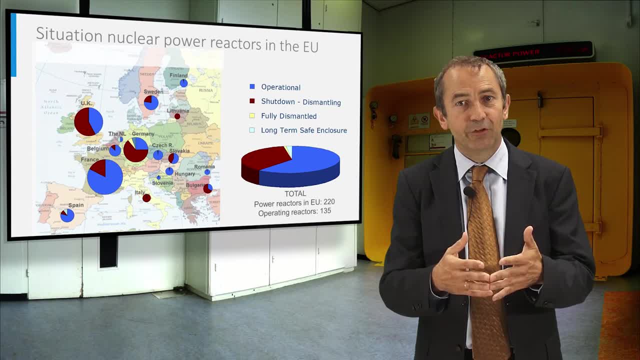 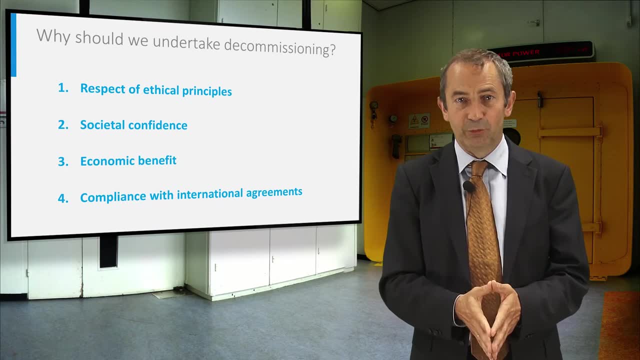 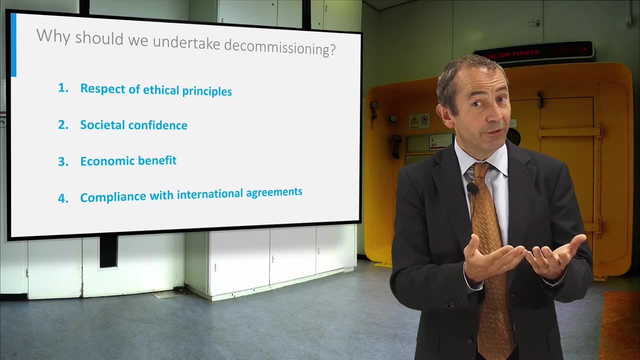 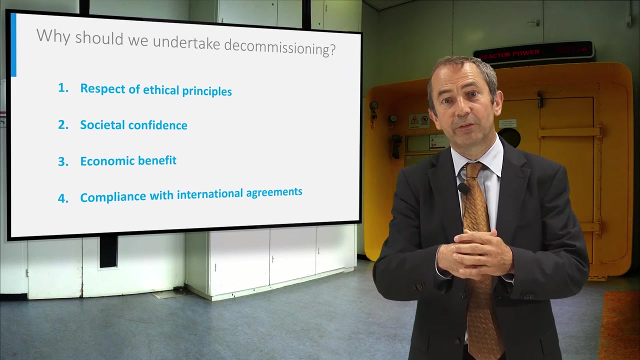 only few major nuclear installations have been fully decommissioned. There are, in my opinion, four principal reasons why we should progress with decommissioning. The first motivation is the respect of ethical principles. Liabilities from past activities may result over time in unacceptable environmental, safety and security risks. 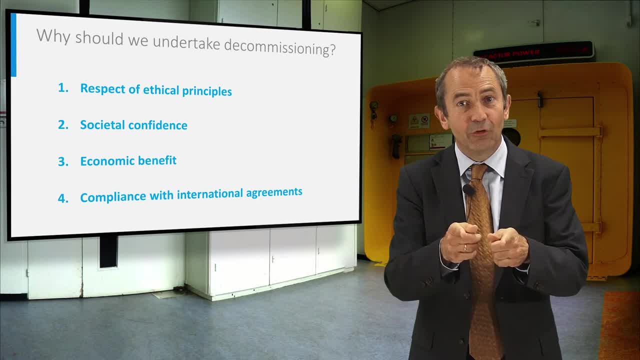 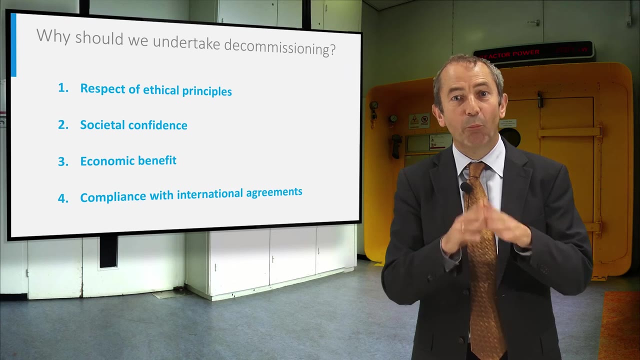 Equity requires that the generation which incurs the liabilities minimizes the burden for future generations. Liabilities should be managed in such a way that potential future impacts are kept at a level that is acceptable both economically and in terms of safety. A second reason is that timely implementation of decommissioning projects 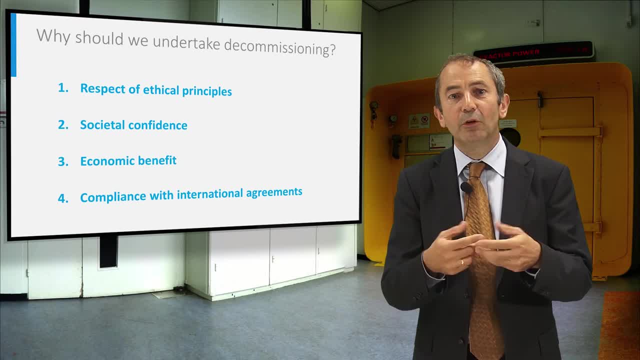 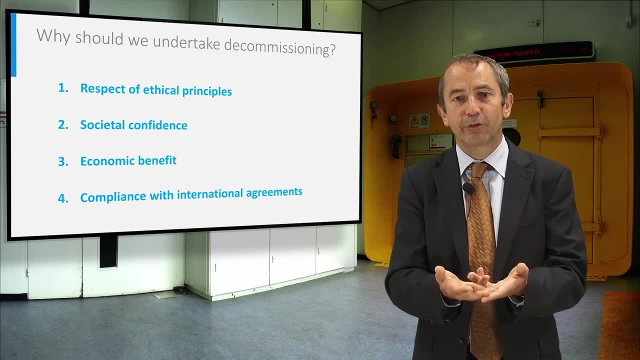 will increase societal confidence in the capability to deal with the long-term consequences of nuclear power, which could facilitate public acceptance for future industrial projects. Complementary to these ethical and societal considerations, there is also an important economic driver for an early implementation of decommissioning programs. 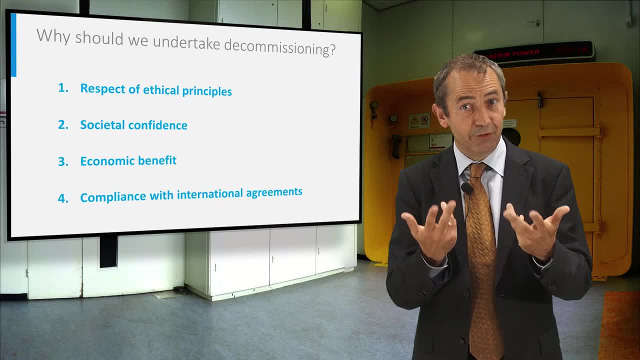 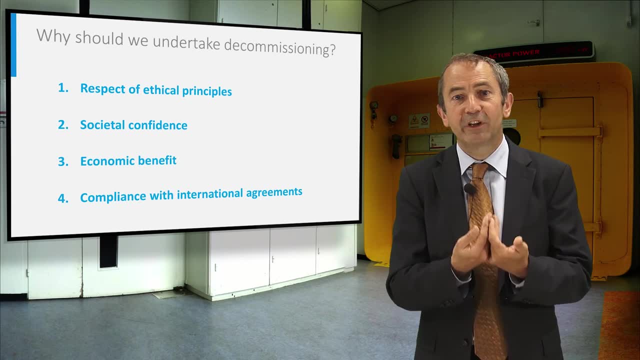 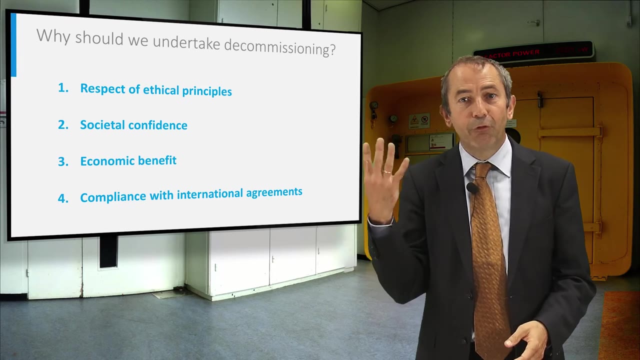 Investments may spur development of new businesses And, conversely, delaying decommissioning projects may be costly due to the potential degradation of structures, the spread of contamination and the loss of knowledge. And the fourth reason is the necessity to comply with international arrangements. 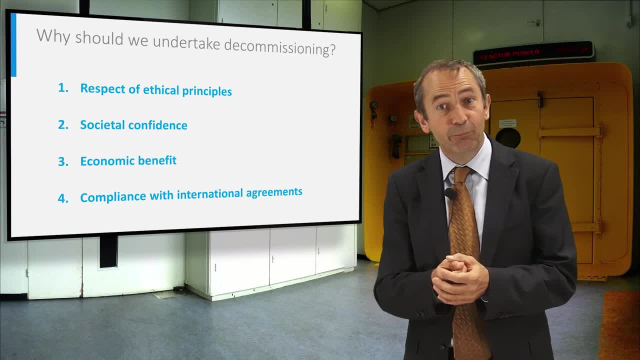 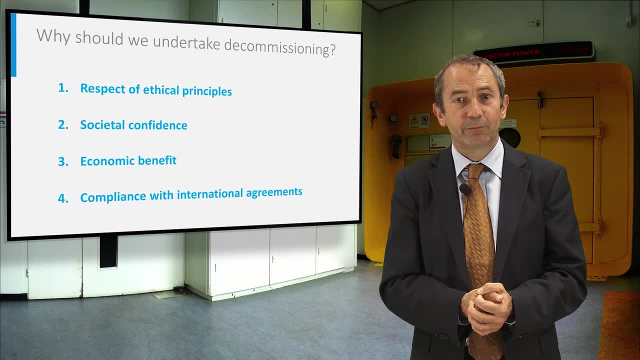 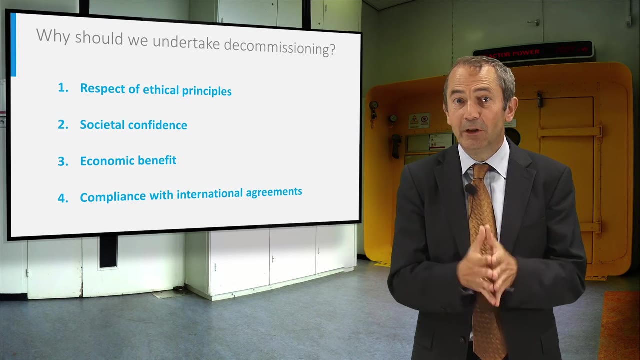 Environmental issues can have a transboundary impact on neighboring countries, and the arrangements made will help to build trust between neighboring countries. Decommissioning is important, but it is not an easy business and the European society faces several challenges. First of all, countries must have a national policy. 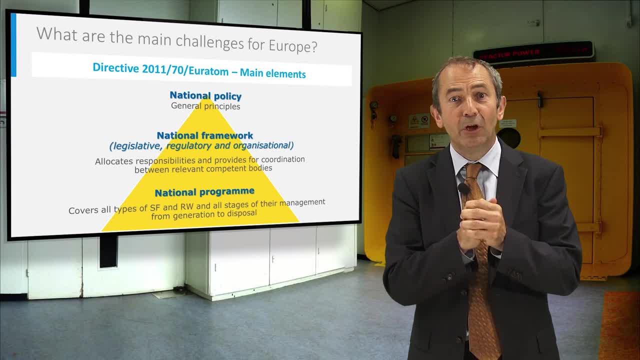 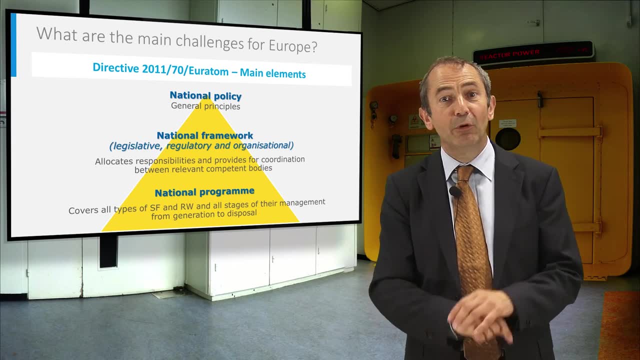 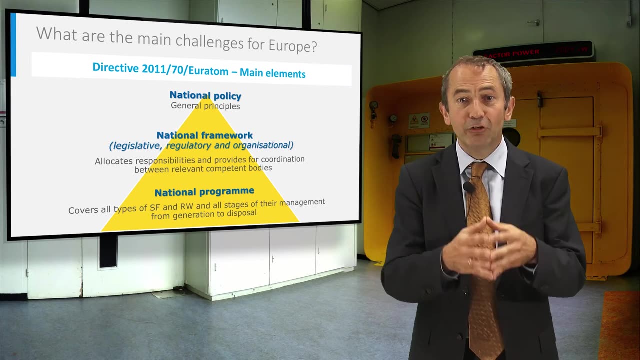 and a supporting framework established to deal with their liabilities. In this sense, the European Directive on the Responsible and Safe Management of Spent Fuel and Radioactive Waste from 2011 imposes to all EU countries- EU Member States- to develop a national program and to report periodically to the European Commission on Evolutions. 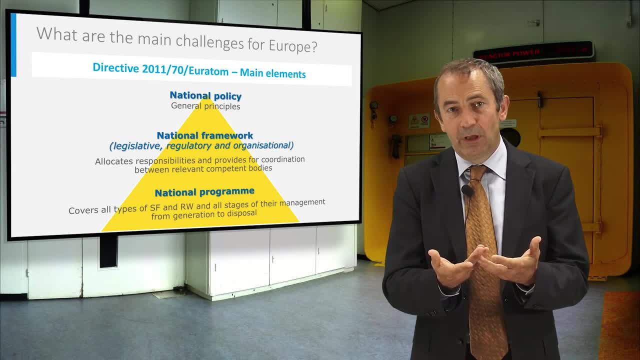 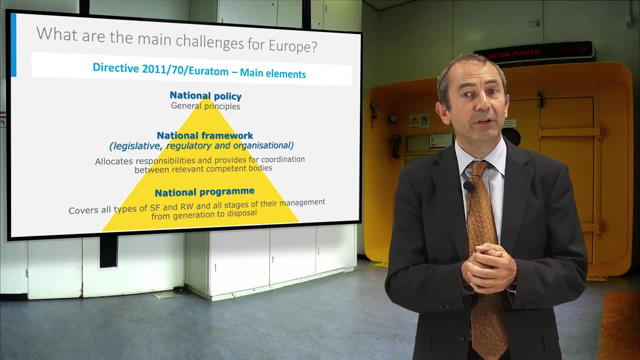 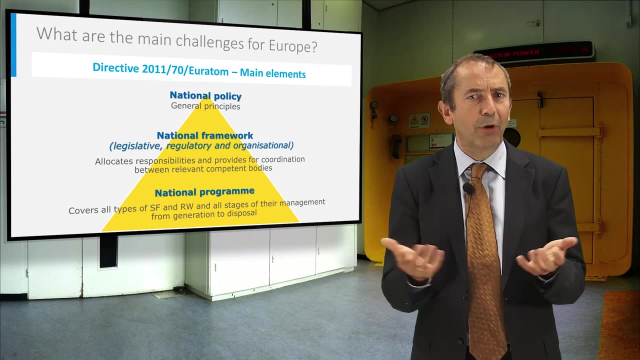 Clearly, decommissioning programs must be financed and EU countries are obliged to ensure reserves. In some countries they are foreseen by the utilities and in others they are counted by a national fund And the commissioning costs estimated for one nuclear power reactor.